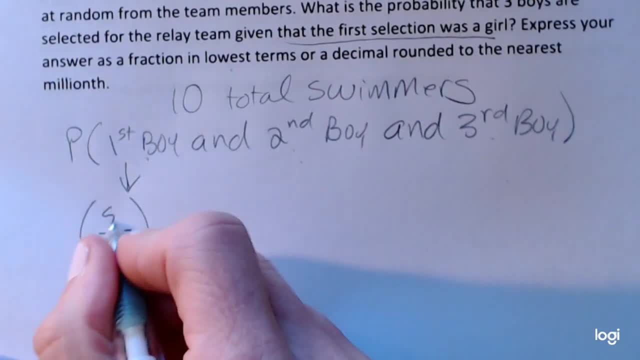 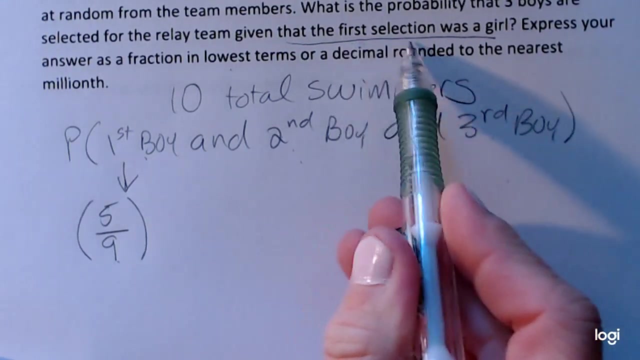 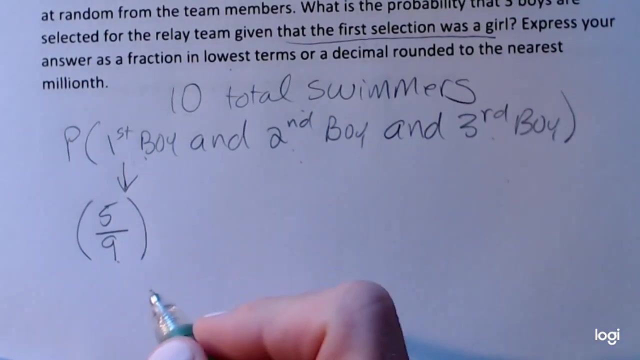 to be okay. I have five boys and ten total swimmers, but a girl has already been selected, so the sample space right here is reduced. I wouldn't put ten in here, I would put nine, because we have already selected a girl. I no longer have ten swimmers to select from. so 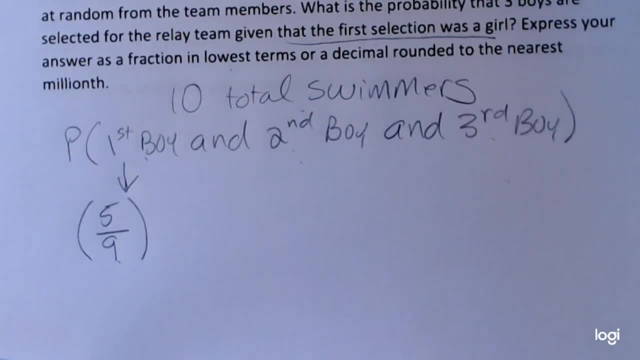 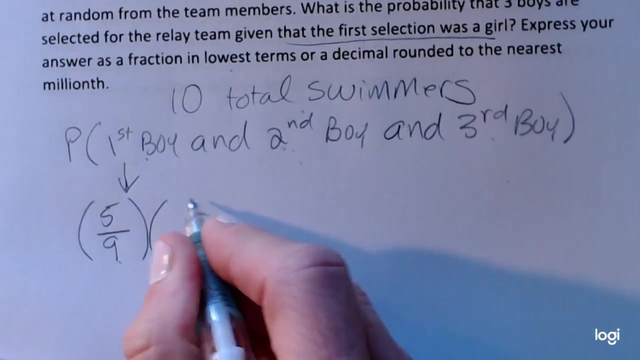 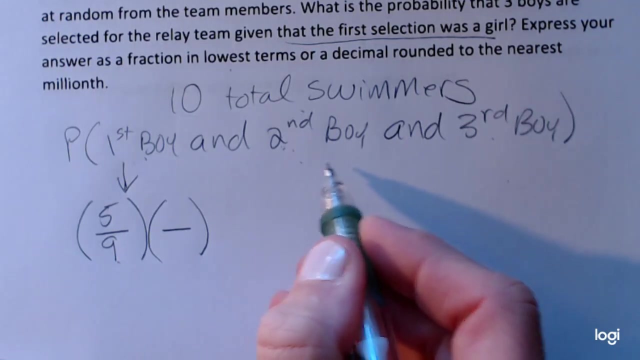 because the sample space is reduced, I necessarily have dependent events. okay, so this is for the first boy. now I need to find the probability that the next selection is a boy, and this is also a conditional probability. it's the probability that this selection is a boy, given that we've already selected a boy and a girl. okay, so the probability. 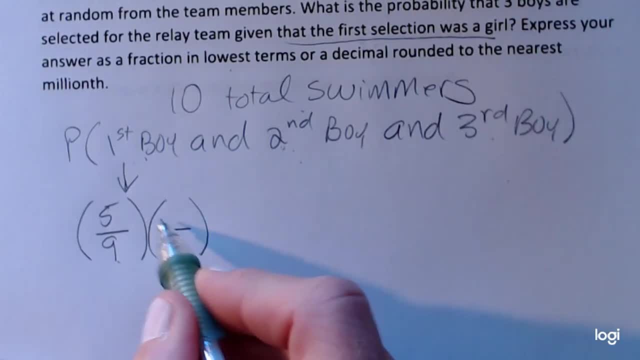 we get another boy here. given that this one was a boy is going to be four out of eight. again, I have to reduce the sample size because a boy has already been selected and then previously a girl has been select, selected. I want to reduce the numerator here because the first selection is: 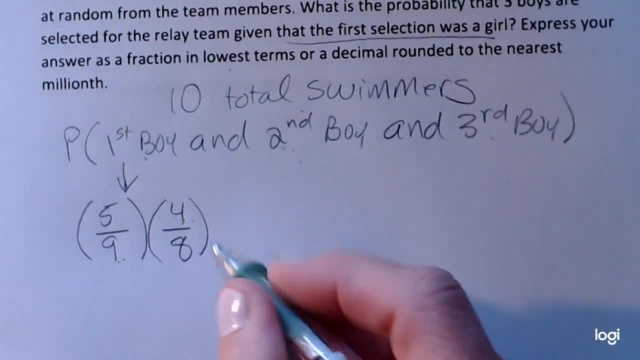 a boy and then the second selection is a boy. so, using the same reasoning again, my sample space will be reduced by one because I've selected three swimmers already and, looking at these numerators, I also need to reduce this numerator by one because two boys have already. 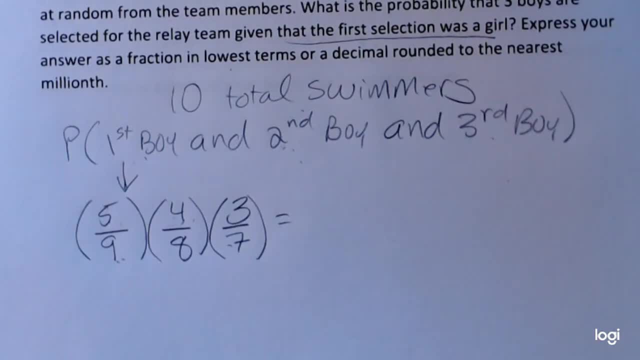 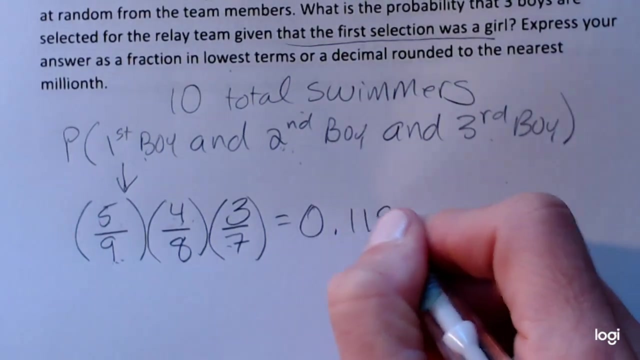 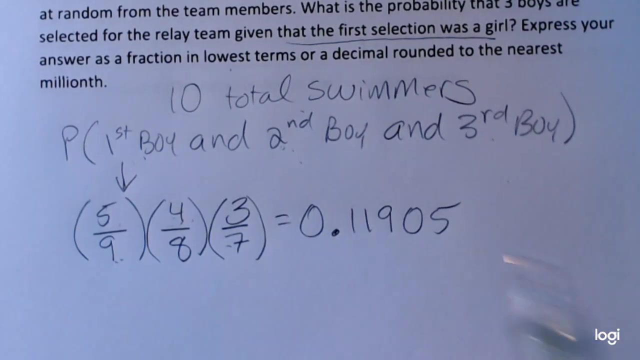 been selected. all right. so once you get that far, the rest is pretty straightforward. it's going to be five times four times three, divided by nine times eight times seven, and rounding to, uh, five. I'll make it exciting. I get about point one one, nine zero five.